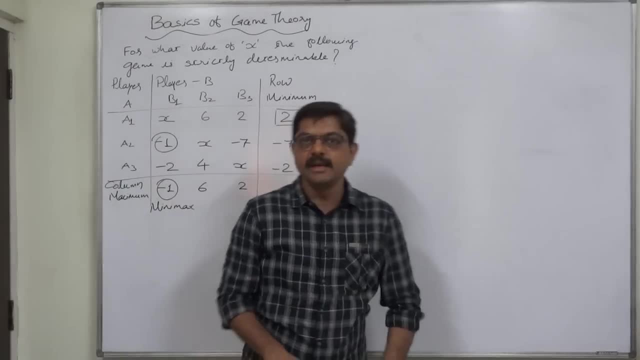 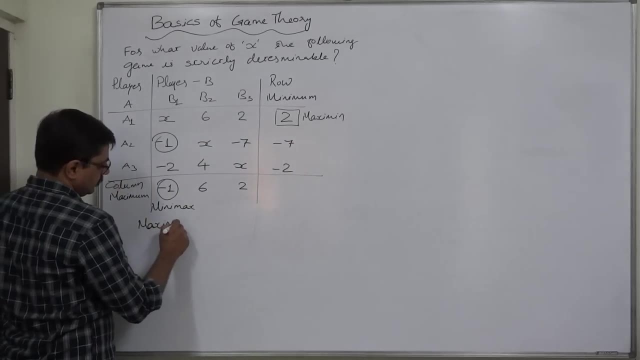 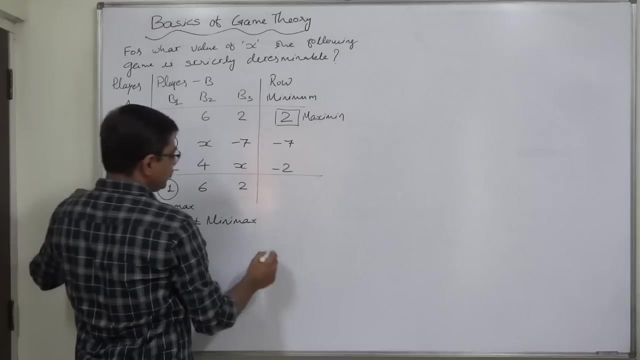 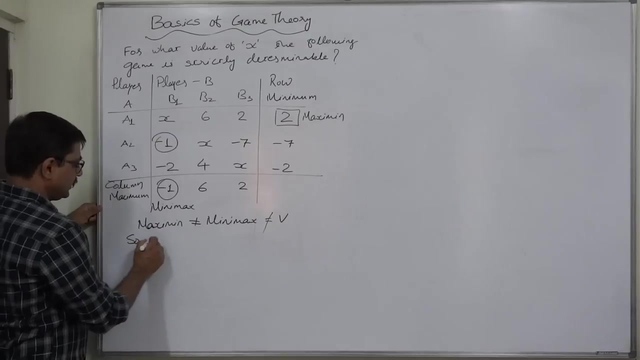 To have the game strictly determinable. maximin equals to minimax, equals to value of game. Here it is not. maximin is not equal to minimax And under such situation we have to take maximin as the value of game. So all the three are not equal. so the game at present is not strictly determinable. 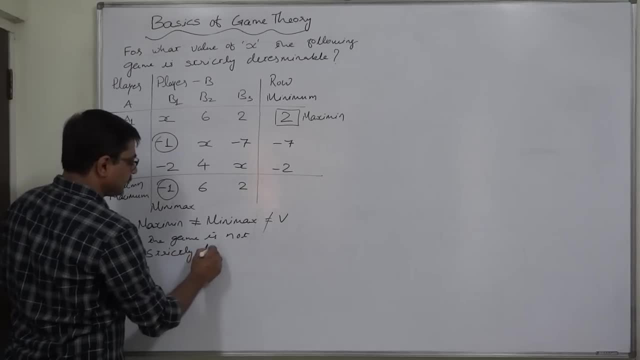 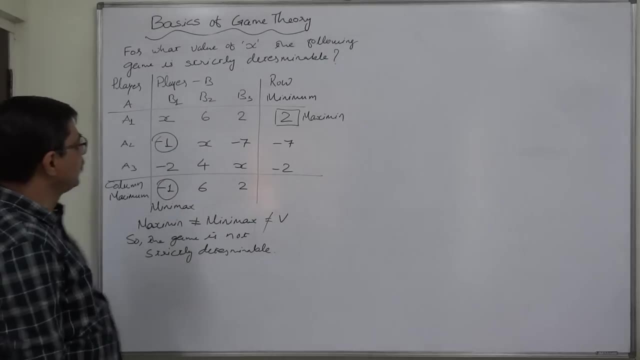 This is the situation at present. Now the question is for what value of x the game can be strictly determinable. The answer is now with us. To have this game strictly determinable, minimax should not be less than minus 1 and maximin should not be greater than 2.. 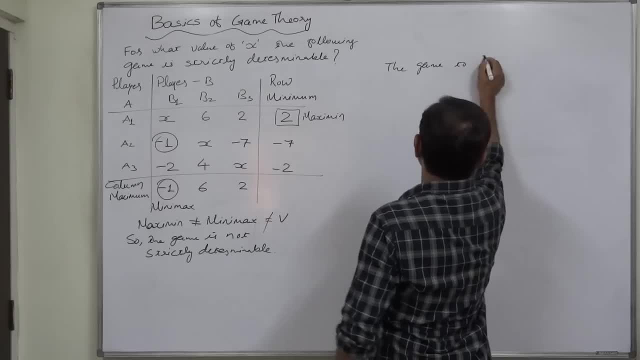 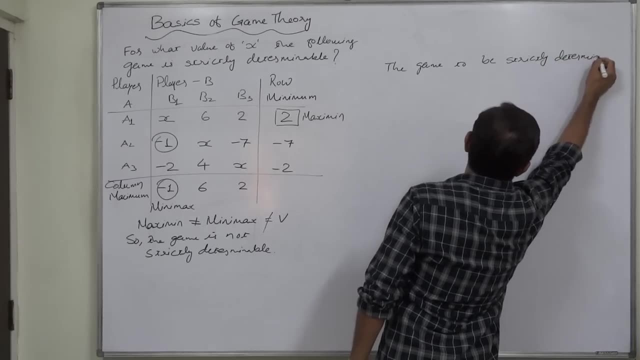 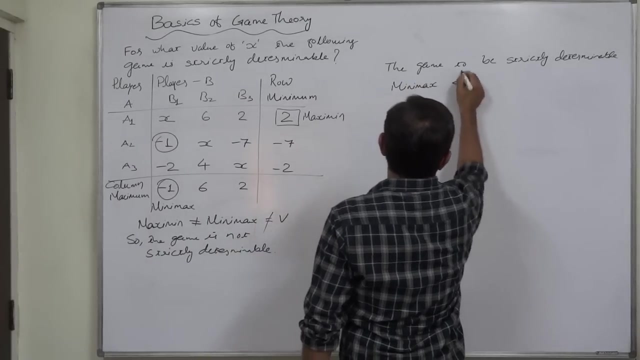 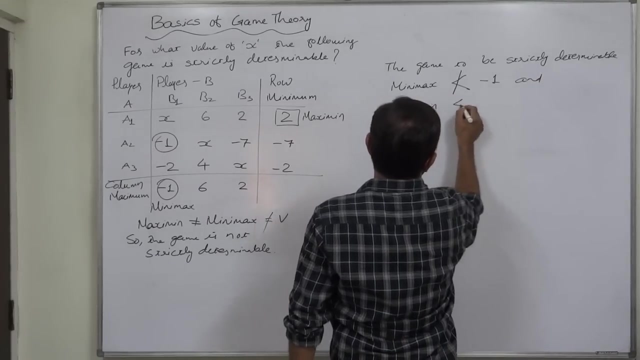 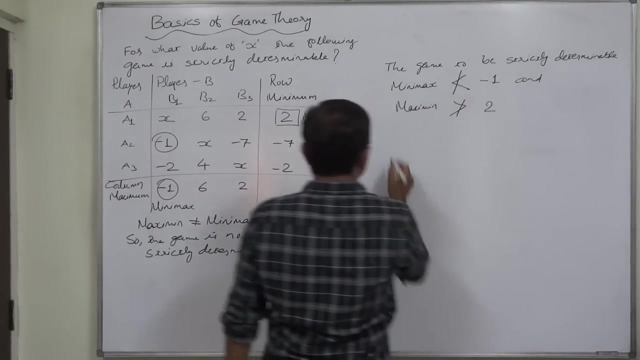 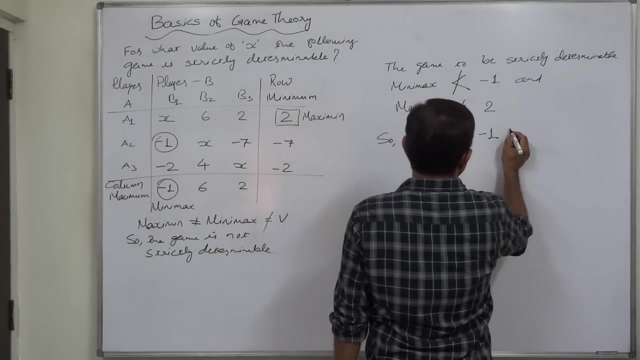 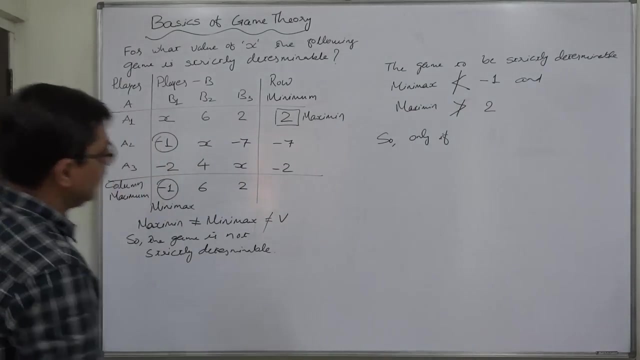 The game to be strictly determinable, Minimax should not be less than minus 1 and, at the same time, maximin should not be greater than 2.. The present values: So only if, so, only if x takes value between minus 1 and 2.. 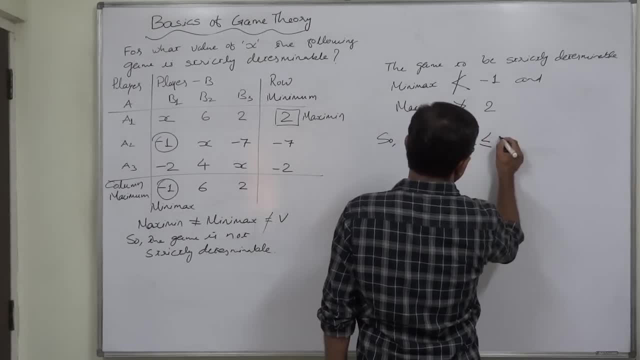 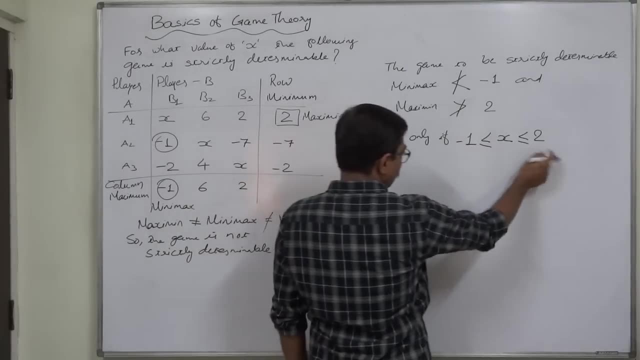 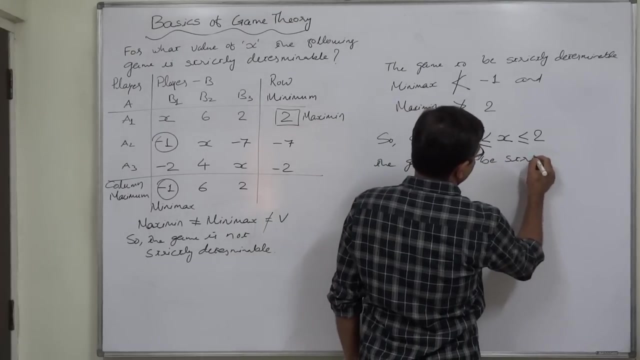 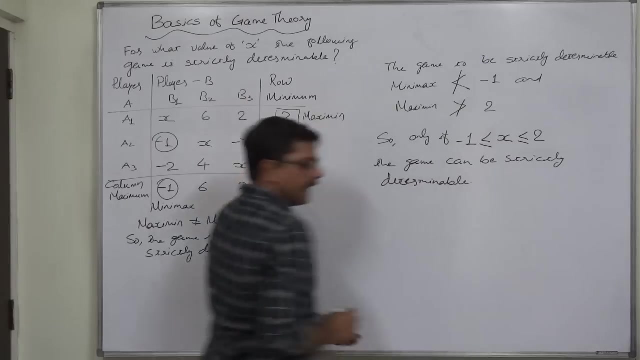 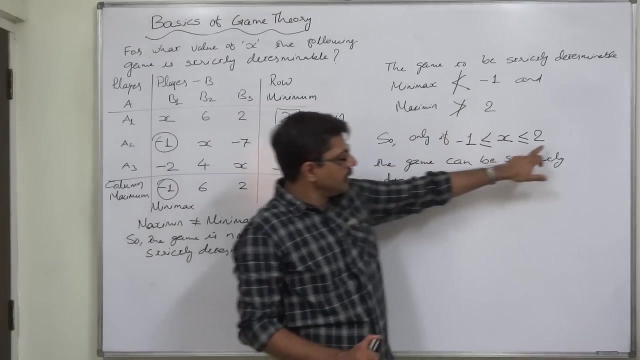 x takes value between minus 1 and 2.. Only if x takes value between minus 1 and 2, the game can be strictly determinable. I suggest you all to assume three types of values of x: One is less than minus 1,, another is greater than 2 and the third is between these two. 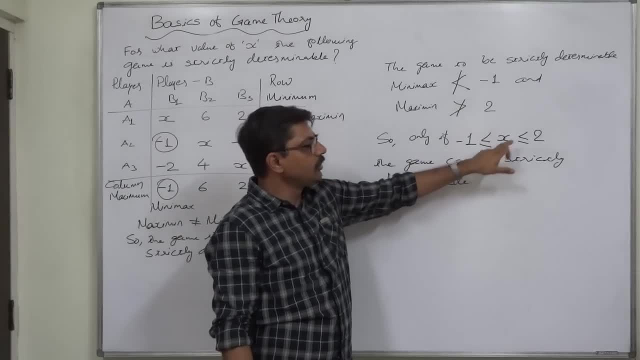 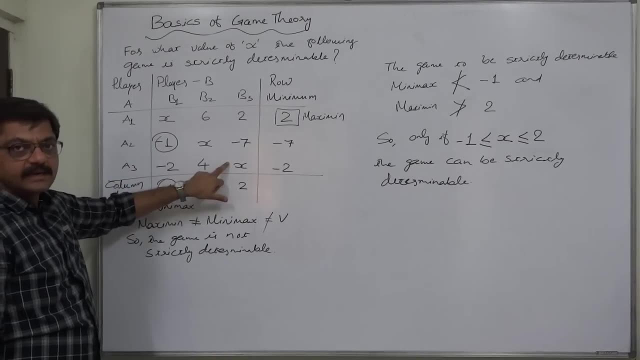 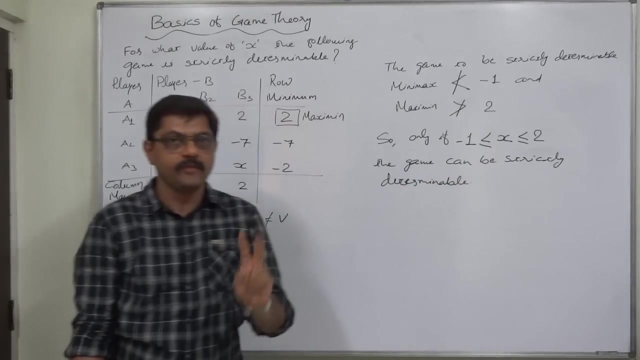 That means any of minus 1 and minus 2.. Minus 1, 0, 1 and 2.. Put them into the matrix at the place of x and observe what happens. This conclusion will be proved valid, But you have to perform three tiles.